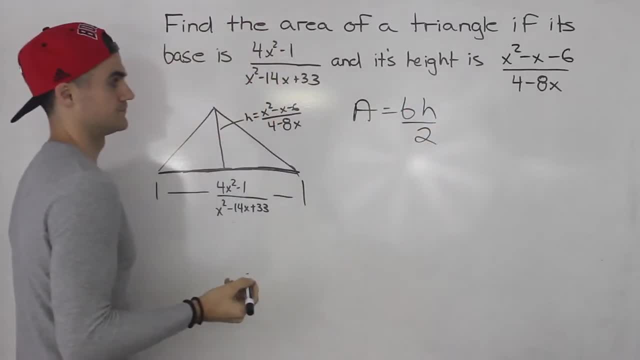 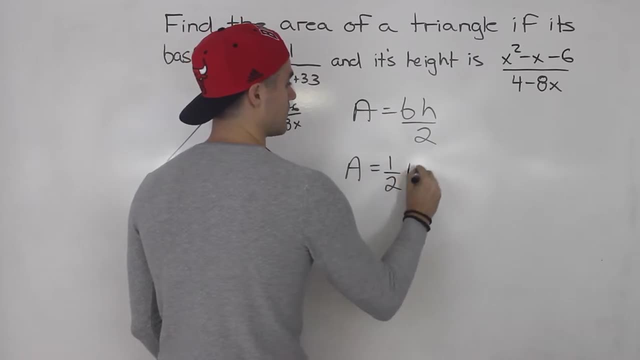 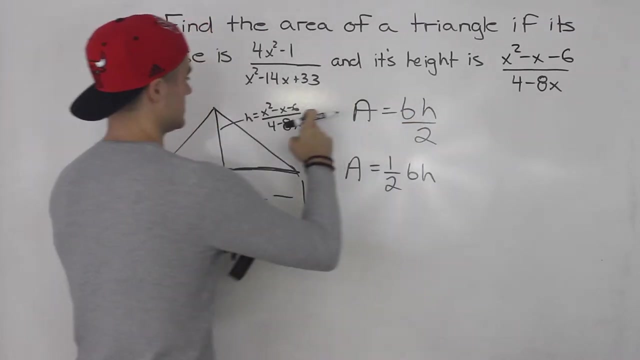 Base times height divided by 2.. And we can actually rewrite this formula. I prefer to rewrite it as: 1. Half base times height, Like that, Because we're going to be multiplying the base and the height, We're going to be multiplying these two rational expressions. So if we're multiplying them and 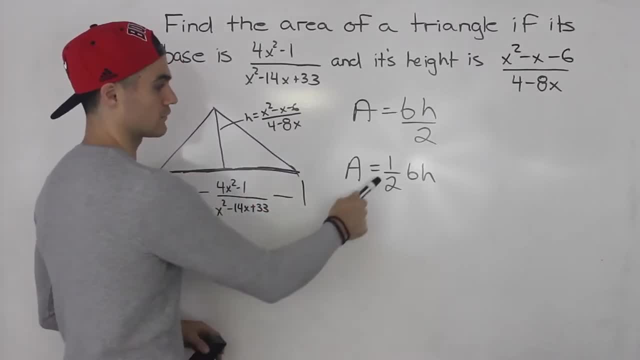 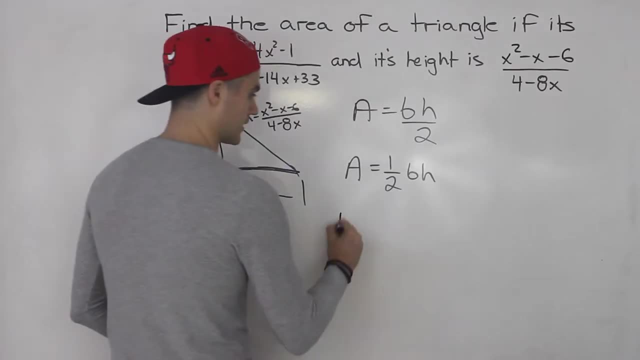 then we're dividing by 2, it just starts to get a little ugly Versus if we put the one half in front, it's going to be a lot nicer. It's going to look a lot nicer. So plugging everything in. 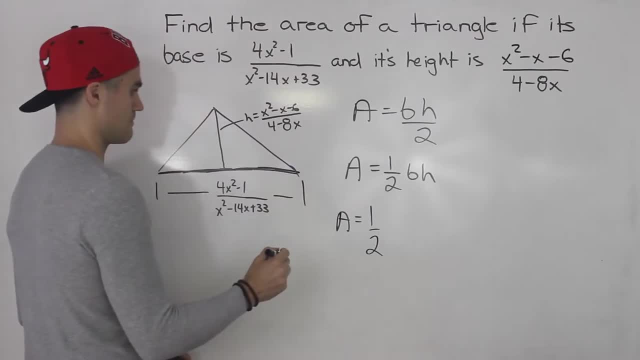 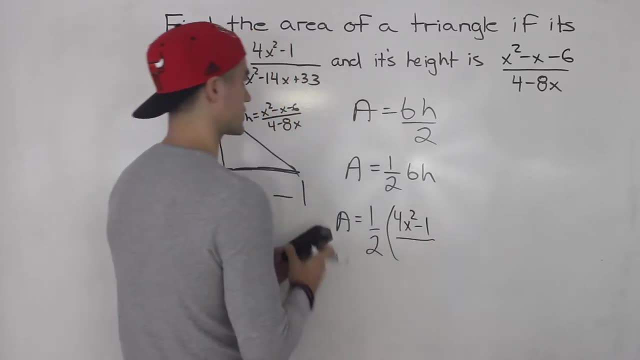 we got one half here. The base is this: 4x squared minus 1.. You know what? actually? I'm going to write this up here, Let's give myself some more room. So basically, the area is one half the base: 4x squared minus 1 over. 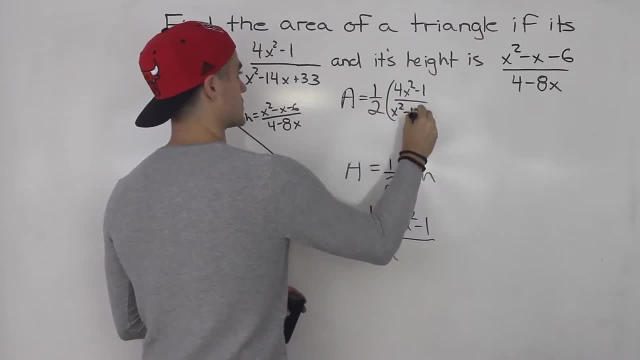 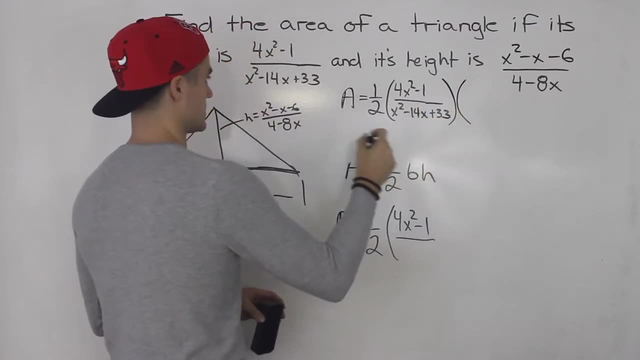 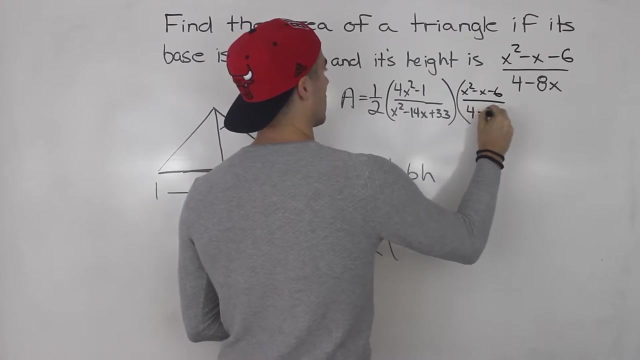 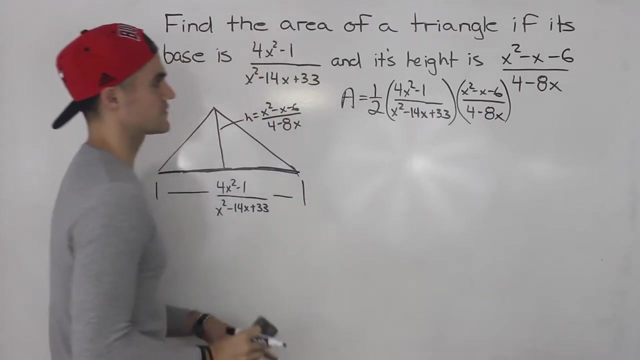 x squared minus 14x plus 33.. And then the height is equal to x squared minus x minus 6, all over 4 minus 8x, like that. So we basically have to simplify this. So we're basically multiplying two rational expressions by each other, and then this one half. 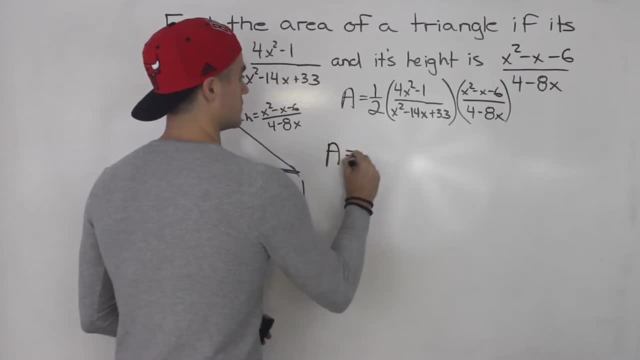 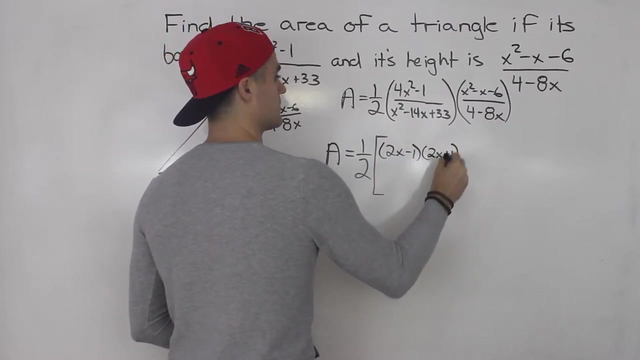 is in front. So what we have to do to simplify is we have to factor everything first. So taking this first bracket, factoring the numerator, that's a difference of squares. that would be 2x minus 1, 2x plus 1 all over x squared minus 14x plus 33. that factors into x minus 3x minus 11.. 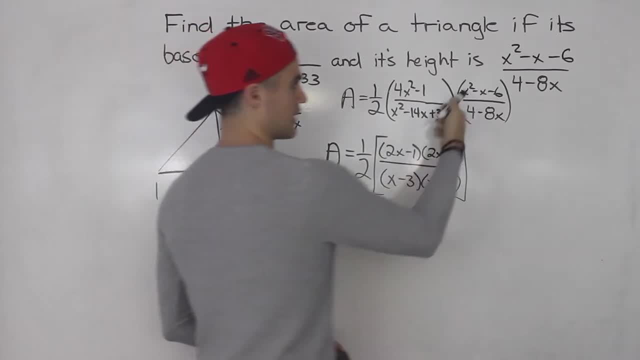 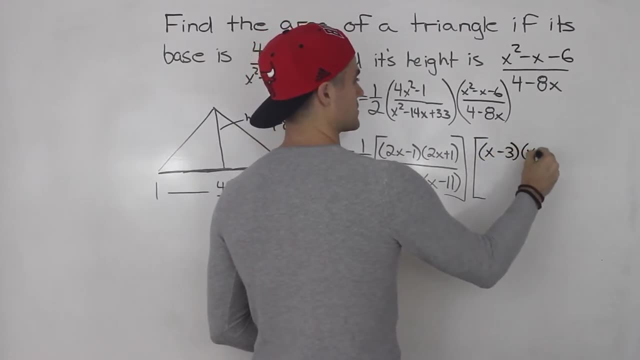 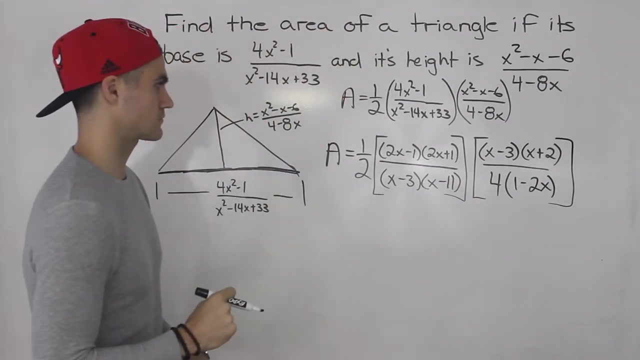 Right. so that is this rational expression simplified. then this one here would simplify to x minus 3x plus 2, and then this one here would simplify to x minus 3x plus 2.. And then from here we could take out a 4 and we'd be left with one minus 2x, like that.